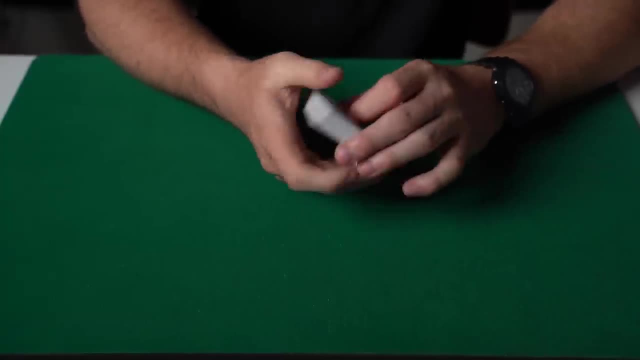 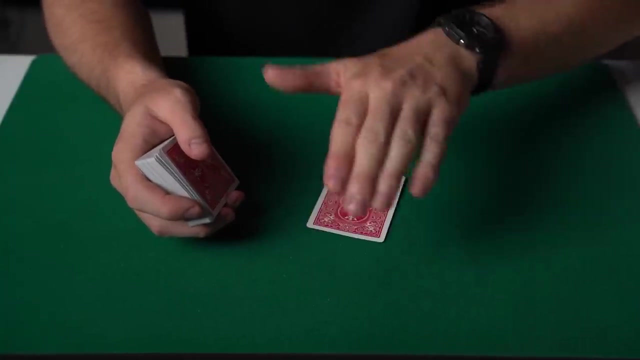 rubbing it into the table. So there are a couple of subtleties that you want to also include to make this more convincing. The first is you want to do a fake rub at the beginning and the card doesn't go through. The second thing you want to do is, as your hand comes over and you pull the card. 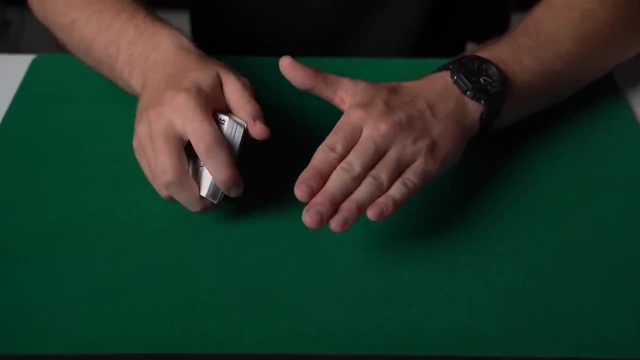 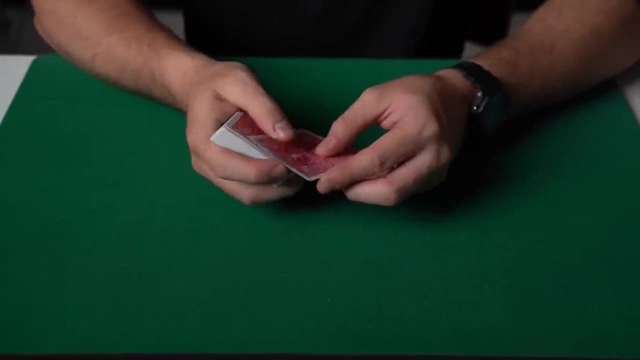 flush. you want to turn your wrist here. Turning your wrist just makes this whole illusion look a little bit more visual and impossible. And then, finally, you want to do a fake rub at the beginning and finally, if you want to be really fancy, you can also have your fingers open. and last second: 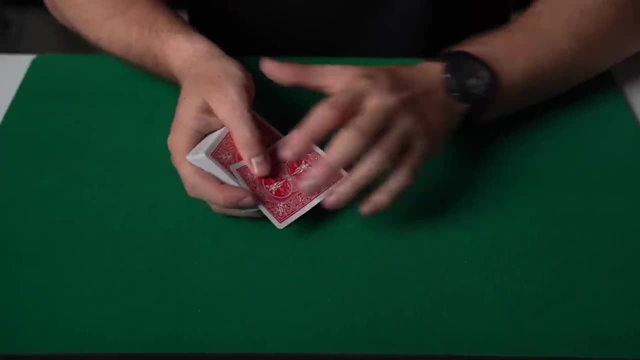 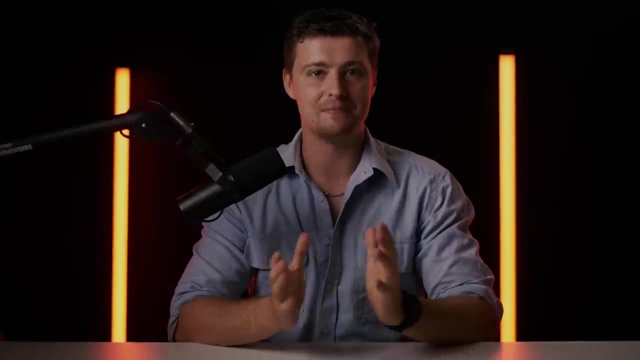 close it and then do the move, And what this does is it just provides more of a retention of the card being in this hand before it goes Very quickly. if you want to learn what I think is the best card trick in the world, then sign up to my free magic webinar. Inside I'm going to be teaching you the 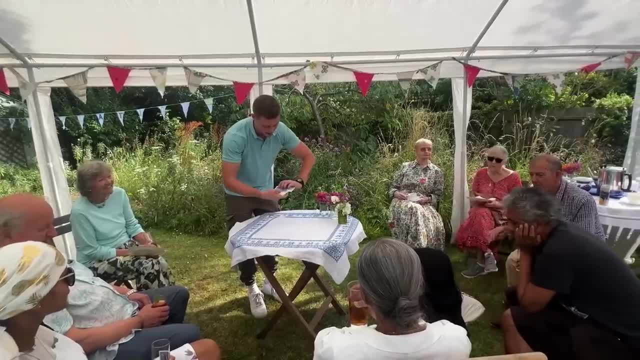 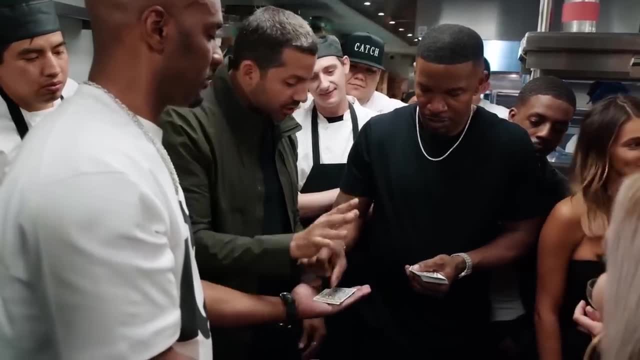 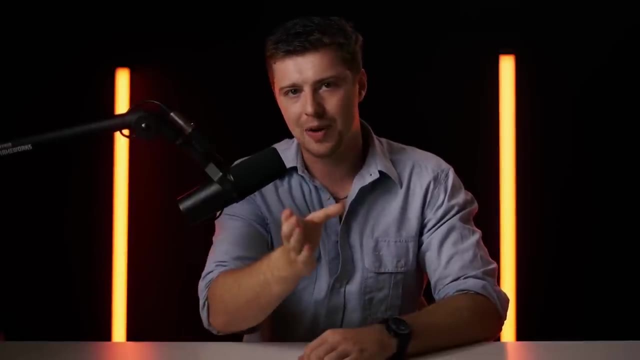 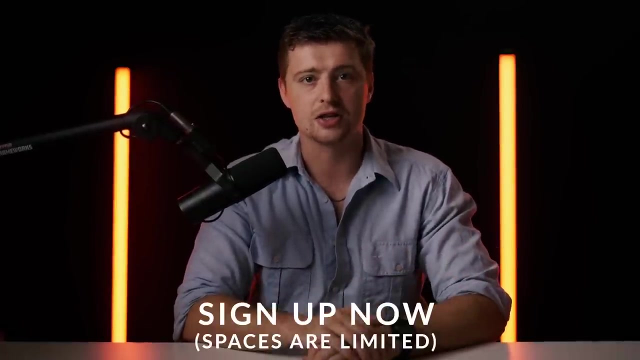 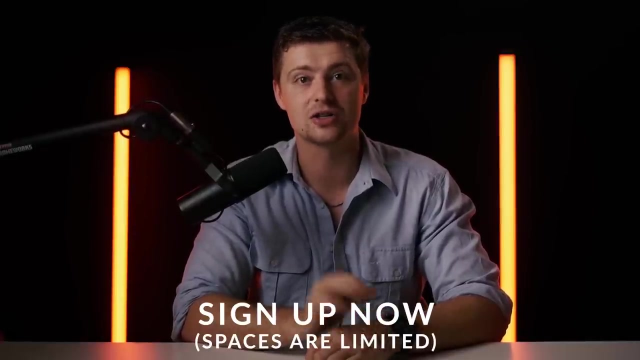 perfect trick to do when you want to amaze your family and friends at something like a dinner party or really anywhere, to be honest. So sign up to one of the free webinars now by clicking the first link in the description. You can also ask me questions live during these webinars so I can help you out. So sign up by clicking the first link in the description, and spaces are limited. So do it now and I'll teach you the best card trick ever to amaze your family, friends and children. 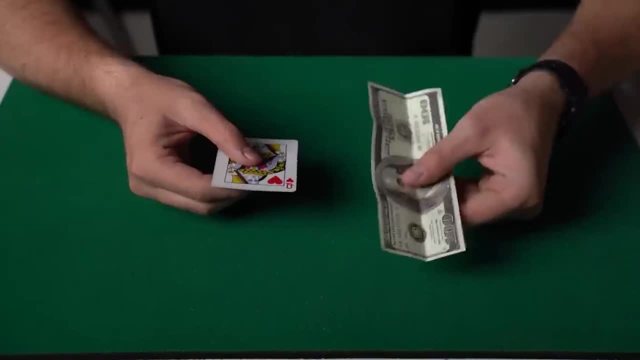 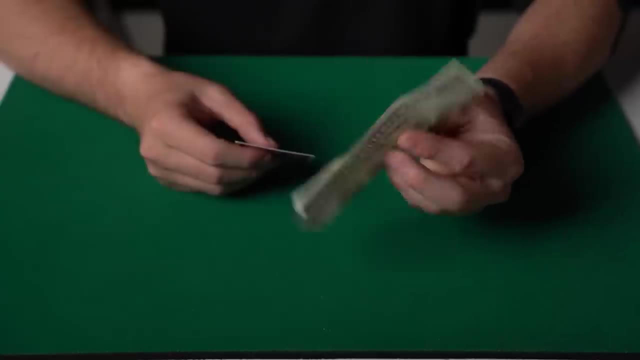 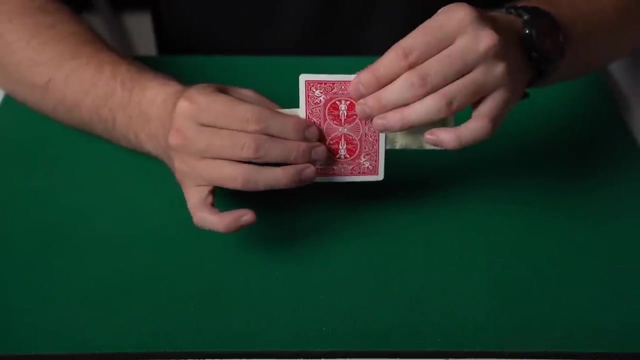 So the magician has a 100% 100 dollar bill and a playing card, And what he does is he takes the money and he folds it up like this, and then he takes the playing card and places it in front of the bill. He then folds the. 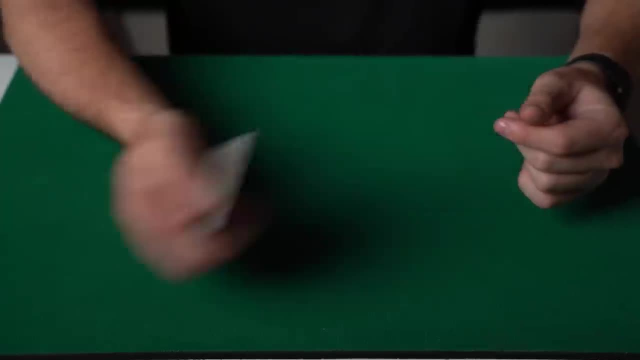 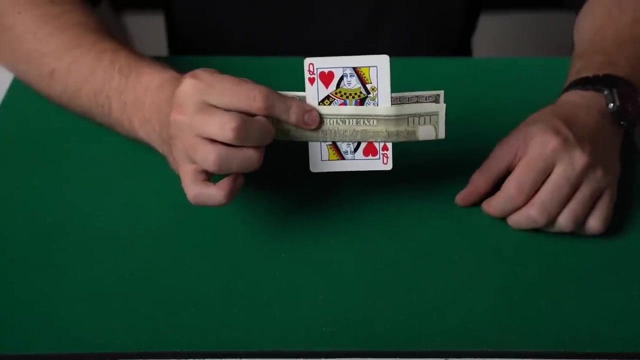 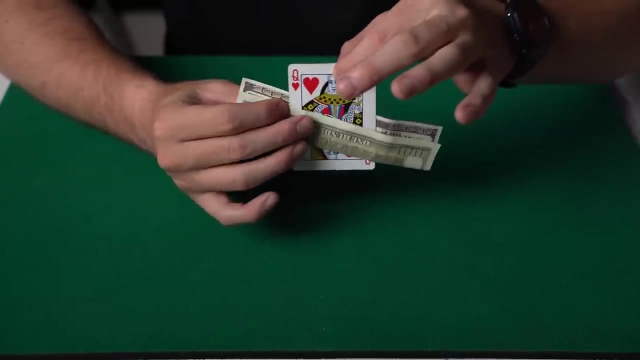 bill around the playing card and when he shakes and waves the card now is melting straight through the bill, just like that. Look how visual that looks. But at the same time he can then even move the playing card around. There we go through the bill as it melts right through the middle of it, and then, whenever he wants, he can. 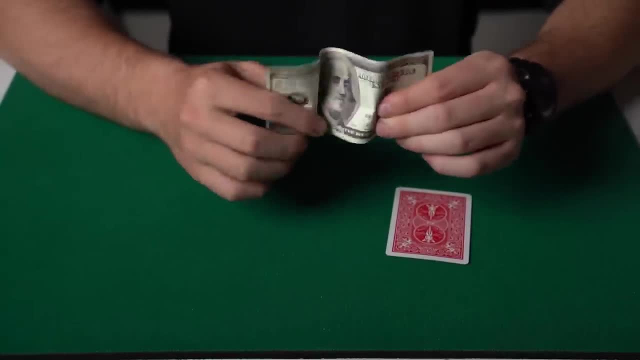 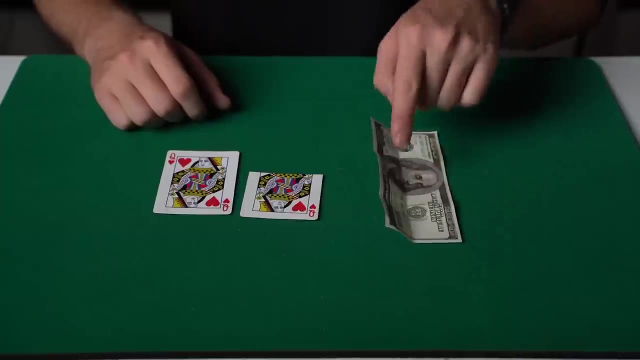 pull the playing card out of the money and hand this note out to be inspected. There are absolutely no holes, as you can see there. For this magic trick you need a paper bill and then two of the same playing cards and one of the playing cards you want to snip off about just under an inch. 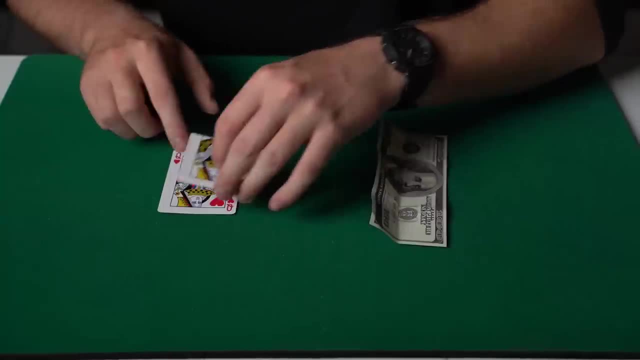 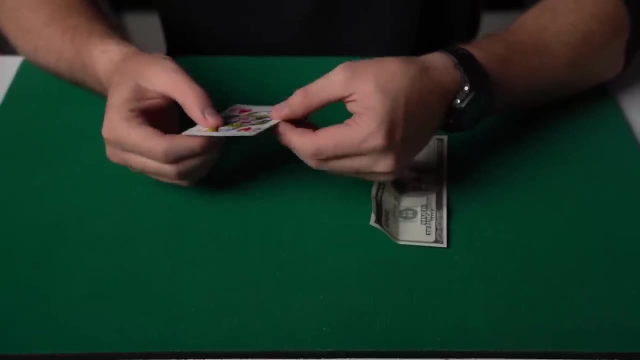 of that playing card, as I've done here. Then you want to stick these two parts together so you can use double-sided tape or glue, doesn't really matter. so it just looks like one playing card. At this point, you want to begin the trick by displaying the bill and displaying the playing. 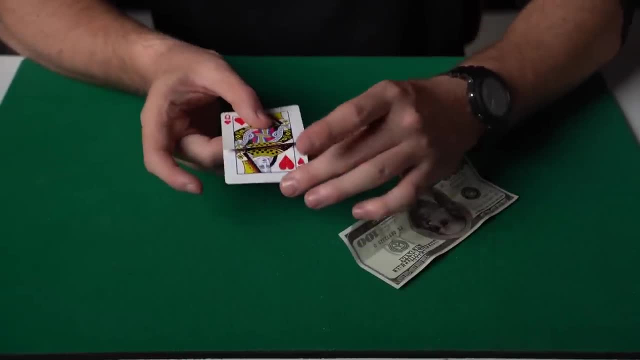 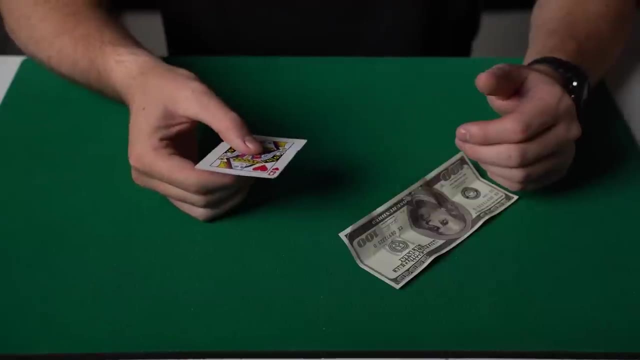 card and you don't want to be holding the playing card this way around because they might see the flap. so you want to hold it closer to you at this sort of angle and it's just very unlikely that you know this looks completely normal and everything's fine. Then what you're going to do. 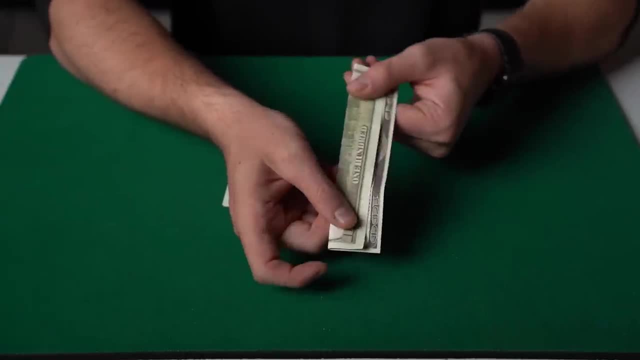 is you're going to fold the bill not in half, but three quarters of the way. and you're going to fold the bill not in half but three quarters of the way, like this, and you want the longest side, the higher side of the bill, facing towards the 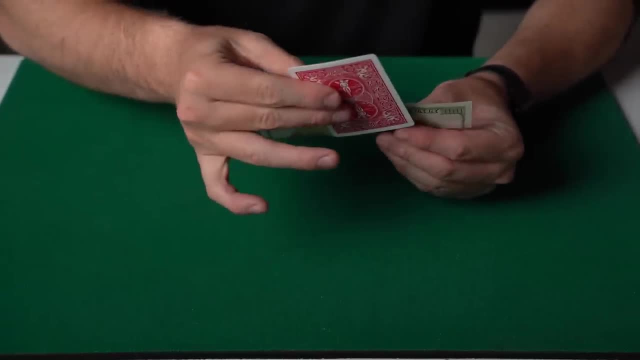 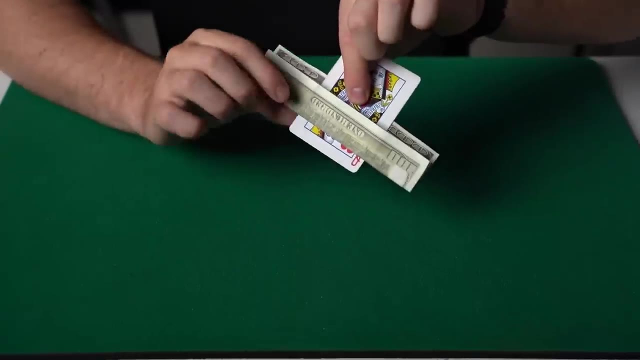 spectator and you're going to place the playing card- what looks like from the front- just in front of the bill. but when you flip it around, what you've actually done is place the flap through the bill like this. so that's what it looks like from the front, but from the back it looks like: 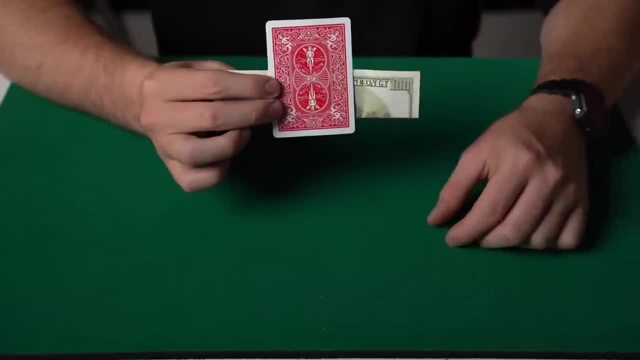 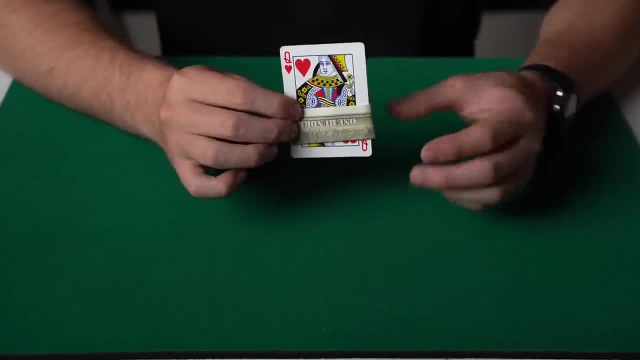 you're just placing the playing card over the back of the bill, Then you wrap the bill around the playing card and you're going to fold the playing card over the back of the bill, Shake and twist, and you now say, look, the playing card has melted straight through the bill. This is 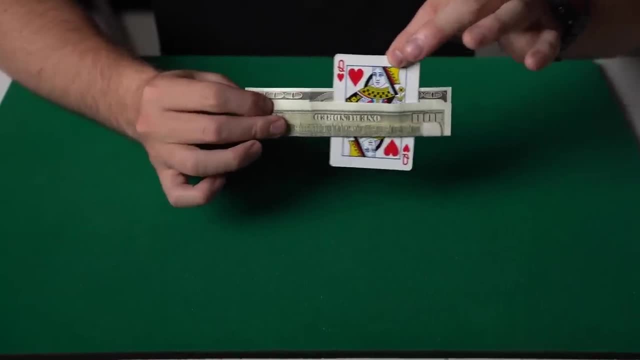 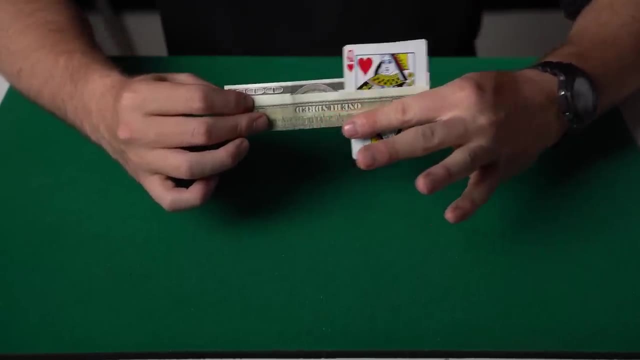 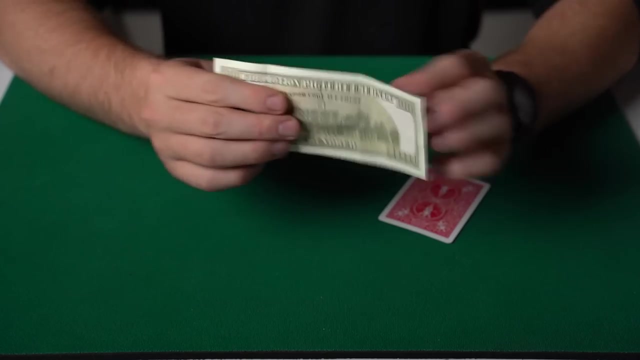 super visual in itself, but then you can actually move the playing card around, move it left, right, up down, and then, when you want to finish the illusion, you just take your finger here, pull the playing card out and drop it onto the table, and then this can be handed out to be inspected. 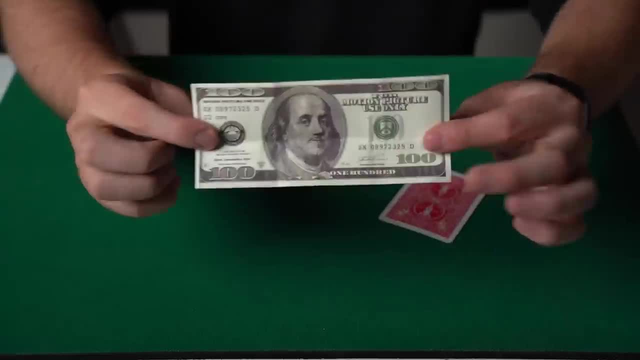 Everyone always thinks that there's something wrong with the bill, like there's a slit or something in it. so you can give this out to be inspected, and then you can actually move the playing card around to be inspected. They look at it, at which point you can put the card in your 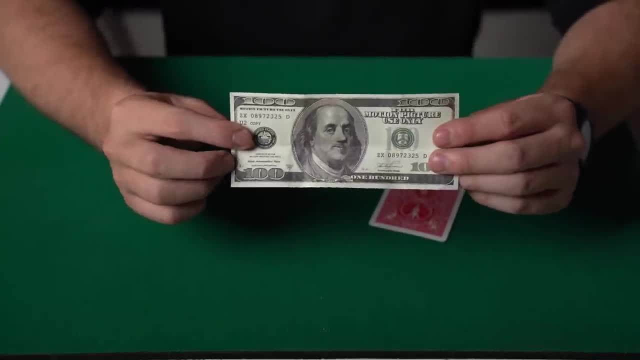 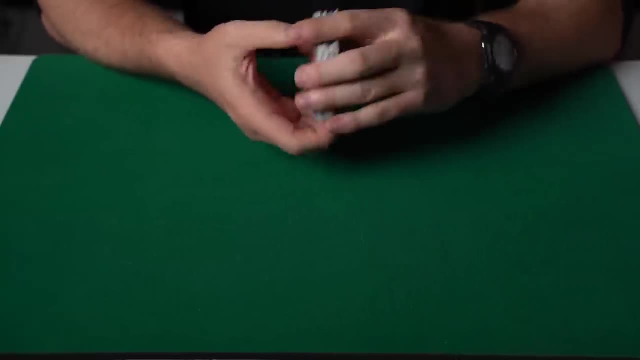 pocket or switch it out for another one. You've got all the misdirection in the world to do that. So the magician's got a deck of cards and he says to the spectator that he wants them to choose one. so he says: say stop, whatever you want. in this case, the spectator's chosen this card here. 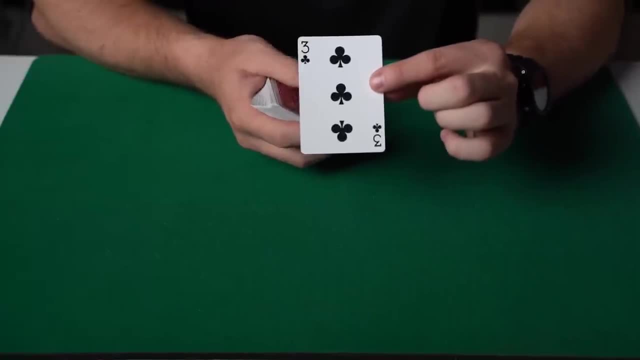 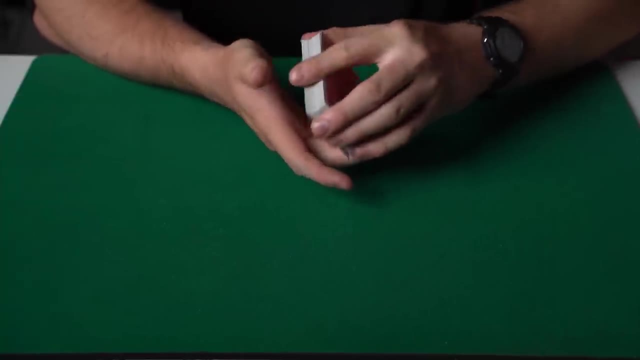 and they're told to remember it. so they've chosen the three of clubs. Obviously the magician wouldn't know this, but he takes back the card and places it somewhere into the middle of the deck, just like that. He then says the spectator's card is going to rise up through the deck and jump to. 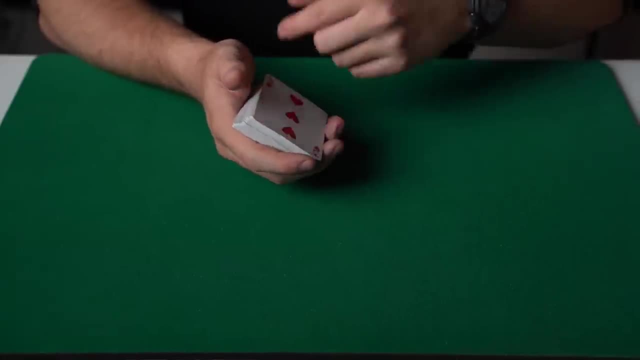 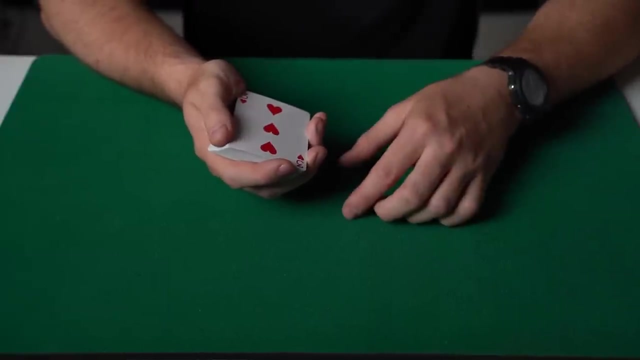 the top. So he snapped his fingers and the spectator's card jumps to the top, which was the three of hearts. At this point the spectator thinks the magician's got the trick wrong because that wasn't their card. so the magician takes it and places it to the side and then says: 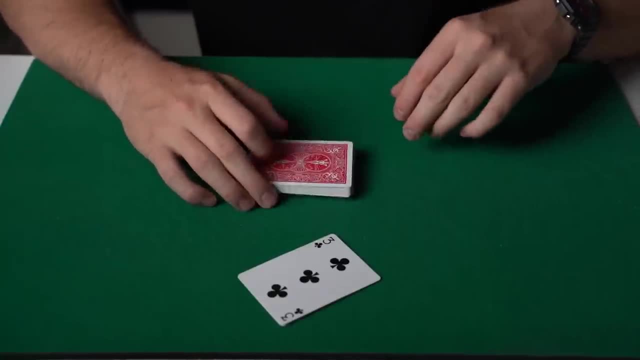 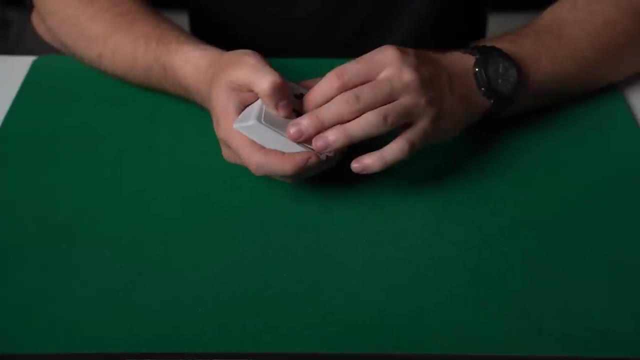 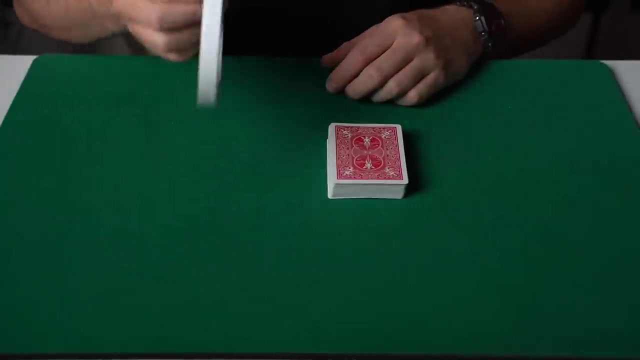 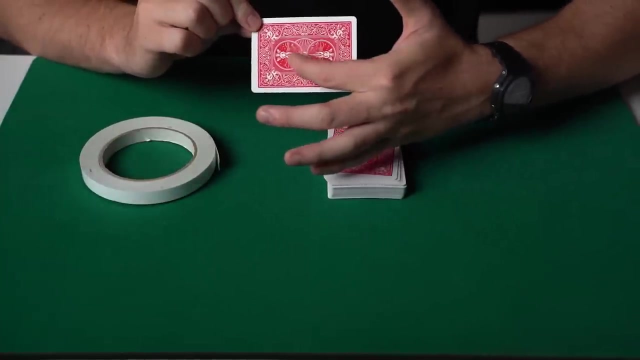 watch this. He picks up the three of hearts, throws it through the deck and it magically changes into the spectator's three of clubs. So this is a very simple effect. that just needs some double-sided tape and then you're ready to go. So take some double-sided tape and just place it here along the middle of the card- only about an 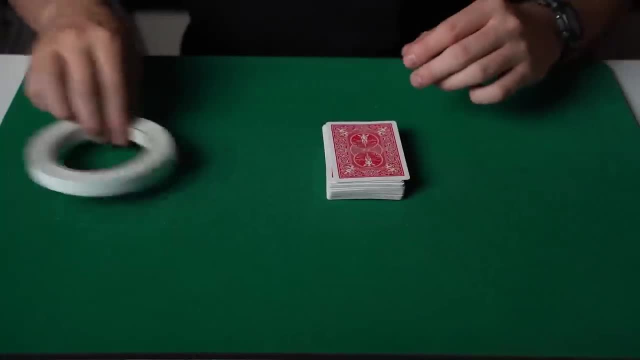 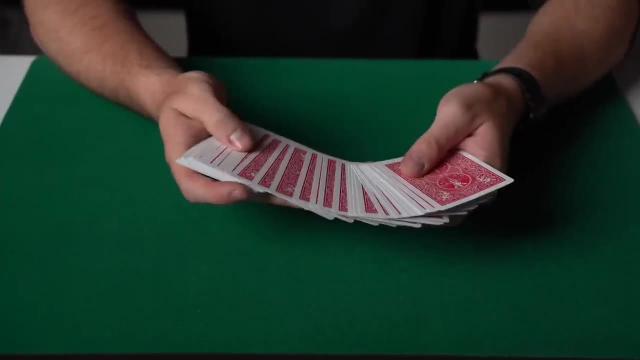 inch or so bang in the center. Once you've done that, you're ready to begin. You can also just get normal tape and double it up, and this will that will also work as well. Then what you need to do is allow the spectator to choose any card that they like, so it doesn't matter if you're going to. 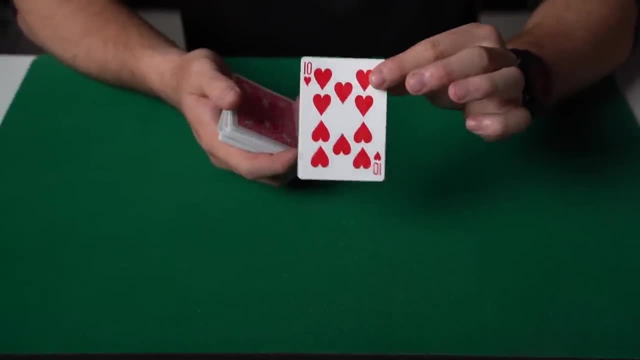 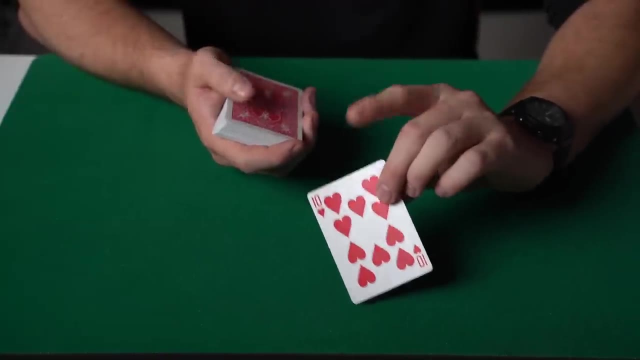 be a ten of hearts and a ten of hearts or whatever. let's just say they choose this card here, the ten of hearts. You're going to show them the card and, as they're looking at the card, you need to do the only slight that this magic trick requires. What you're going to do is known as a Marlow tilt. 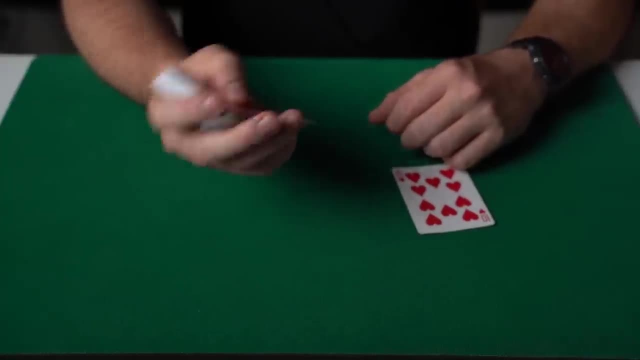 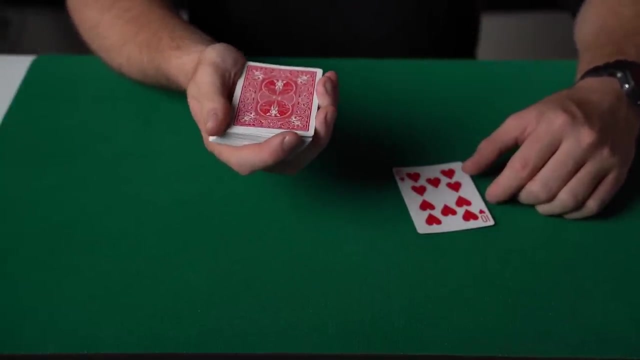 which is where you push the top card to the side and you pull it back, but you stick your little finger under it. So that's what the Marlow tilt looks like. I'll just show you that again. You hold the cards like this: You push the top card to the side, You pull back, You pull the top card. 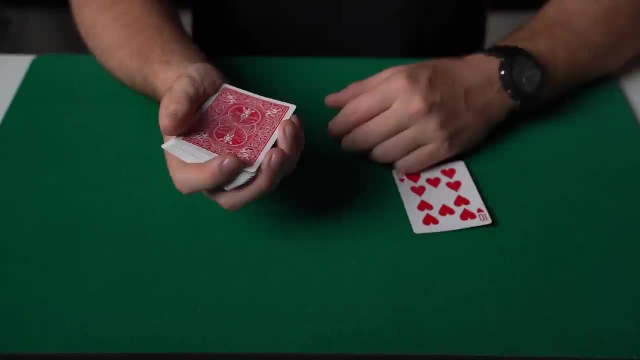 back. You pull the top card to the side. You pull back, You pull the top card to the side, You pull, and now my little finger is under the top card. Anyway, just practice doing this for me now. Hold the cards like this with your thumb along one edge, first finger. 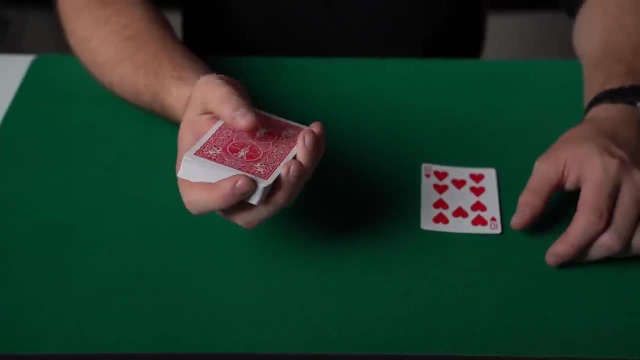 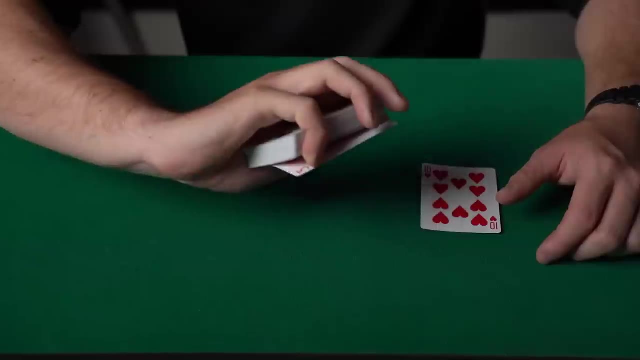 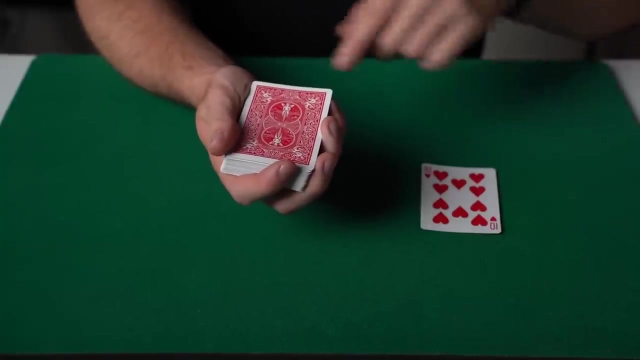 across the top and these three fingers on the side then use your thumb to push across the top card and then you pull back with your thumb and you see how my little finger is now underneath the top card. What this does is it creates something known as a depth illusion, where it looks like the deck is.